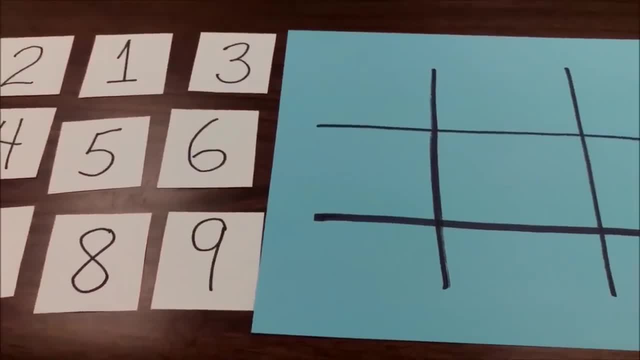 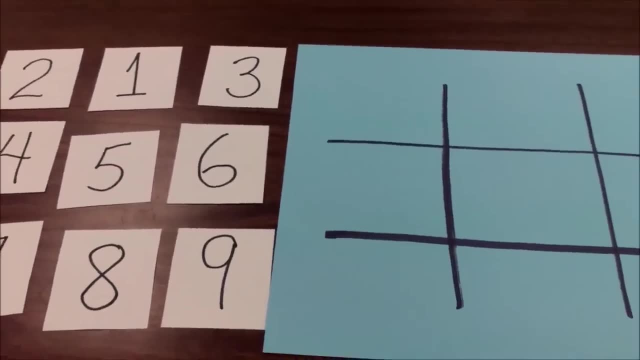 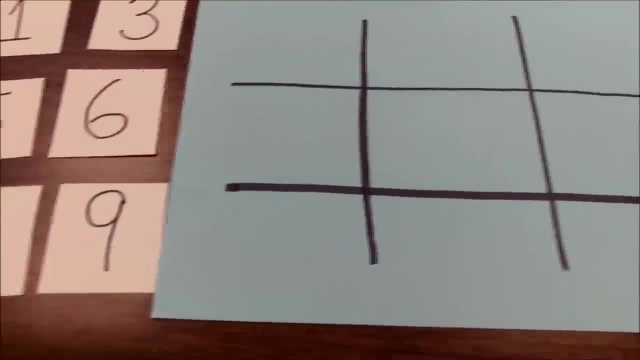 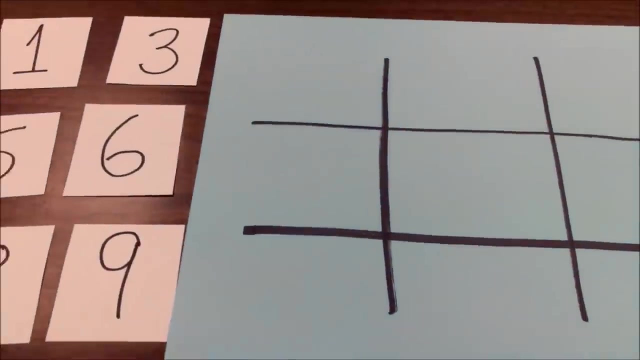 This is a pretty cool game. It gets kids to really think and think sequentially, think ahead. Just a good problem solving game, And it's a fun and easy game too. So what we have is we have a tic-tac-toe game board here, And then we have numbers 1 through 9.. Basically, it's like regular tic-tac-toe, except- here's the kicker for you, those that are into math: 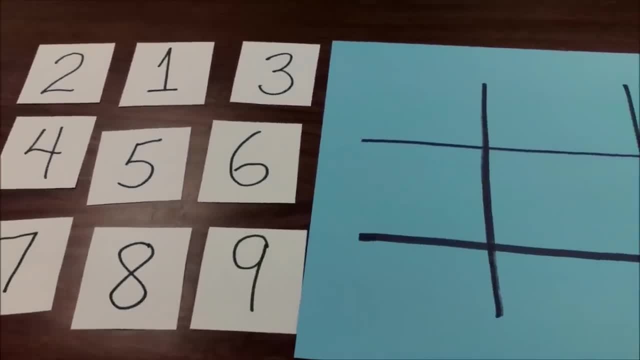 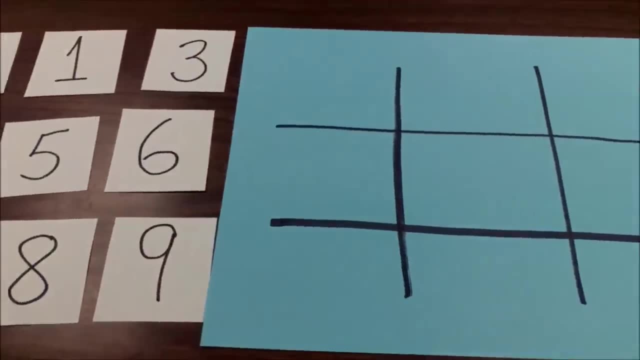 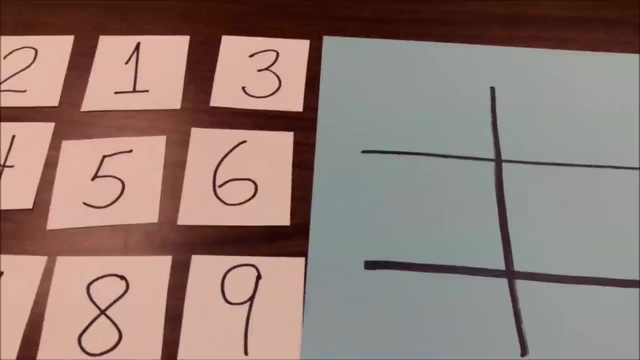 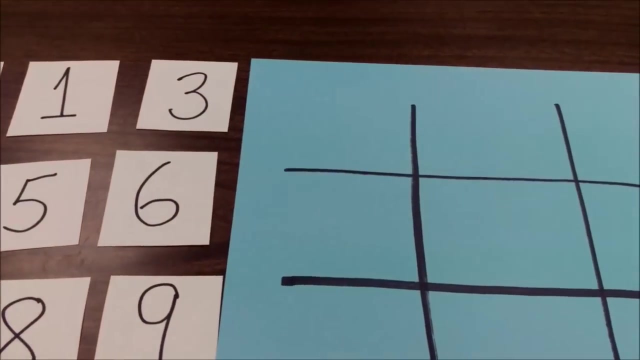 To win, you want to be the person who places the third number in a column, row or diagonal to add up to 15.. So let me just kind of demonstrate how this would work. You take turns. you know you can rock paper scissors to see who goes first. There's one rule for the person who goes first is that they cannot put a 5 in the middle. 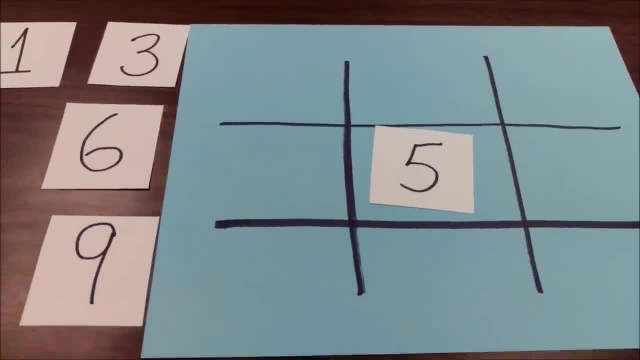 And you can go ahead and do that. You can ask Mr Hino, why can you not put a 5 in the middle? Because if you do, it guarantees that you're going to win. I don't know, it's kind of like cheating. 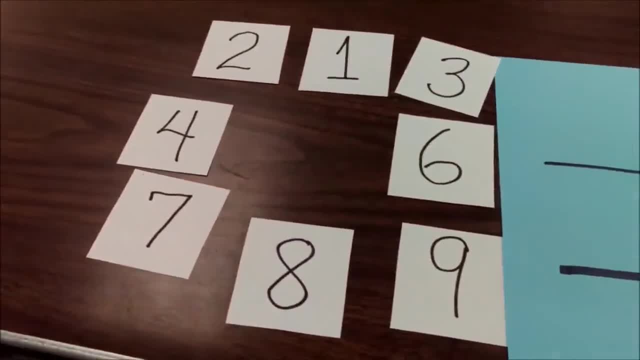 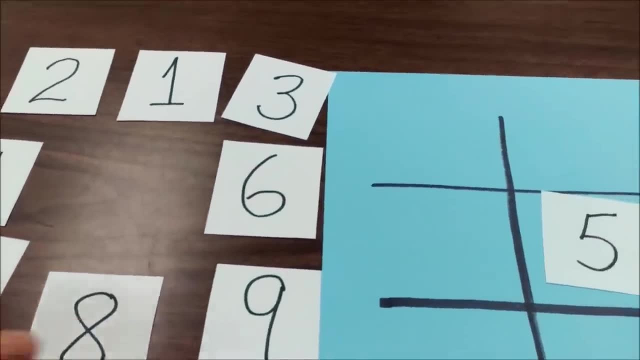 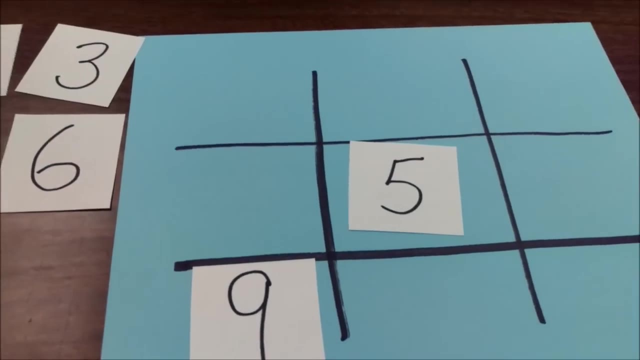 Because, look, if you put a 5 in the middle and the next person puts a number, there's nothing they can put that keeps you from not winning. if that made sense. I mean, look, if you put a 9 here, then the next person that puts a number, all they got to do is put a 1 up here. 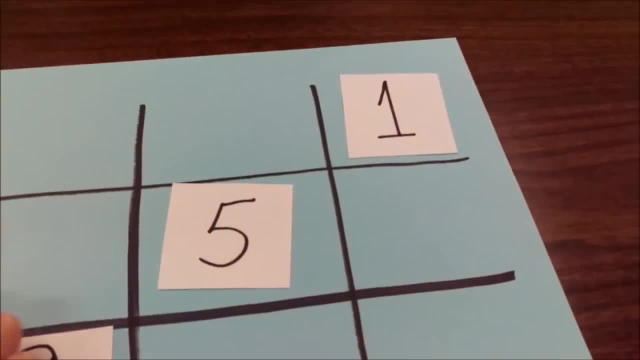 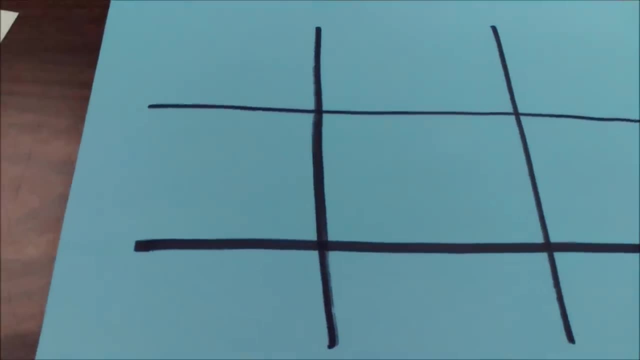 And they win. That equals 15.. So that's one of the rules: You just cannot put a 5 in the middle. to start with, You can put a 5 anywhere else, but you just can't put it in the middle. 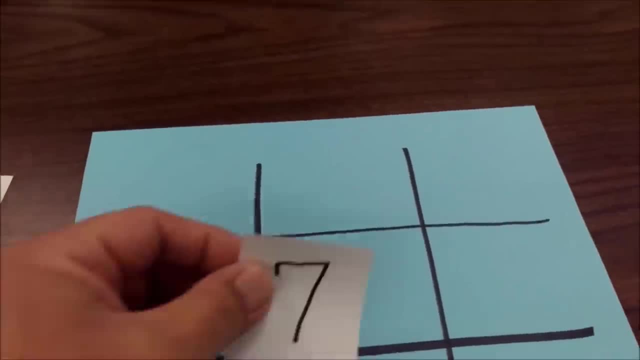 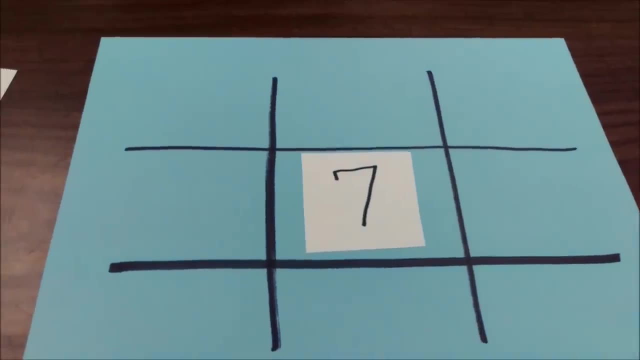 So let's just pretend we're playing a game. So let's say I go first and I put a 7 in the middle. Strategy would say: well, I have to make sure I don't put a number, if I'm going to put a number in. 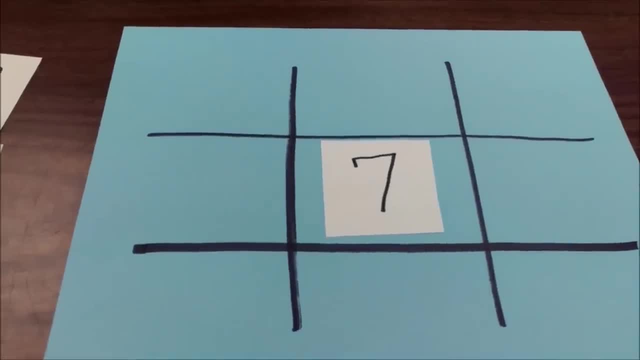 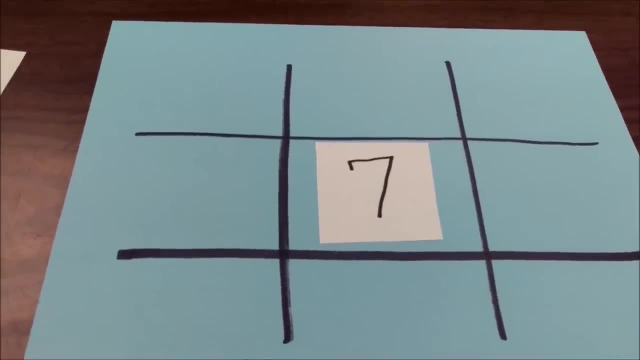 And right now, if I put a number, I'm going to have to put a number down in 7's column row or diagonal, because there's just no way around it. So one strategy would be okay. I'll put a 9 here. 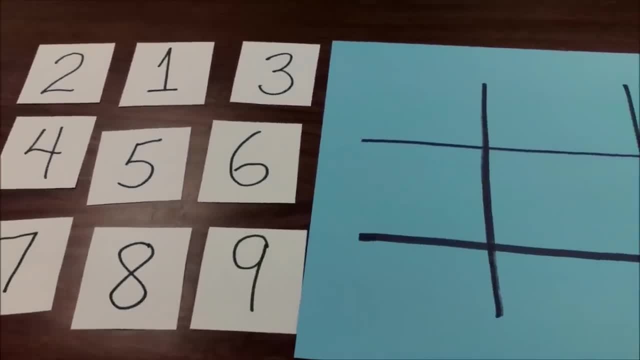 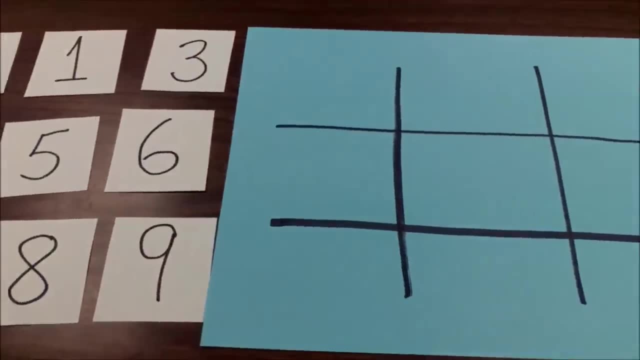 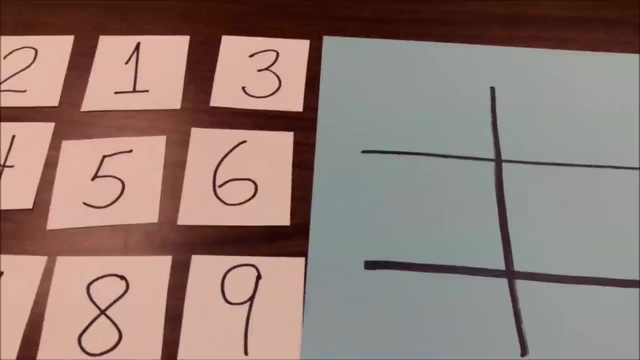 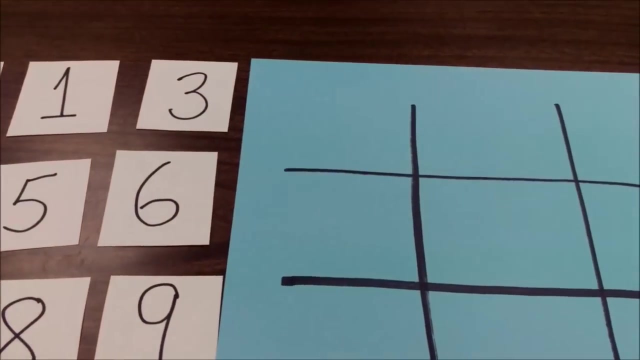 To win, you want to be the person who places the third number in a column, row or diagonal to add up to 15.. So let me just kind of demonstrate how this would work. You take turns. you know you can rock paper scissors to see who goes first. There's one rule for the person who goes first is that they cannot put a 5 in the middle. 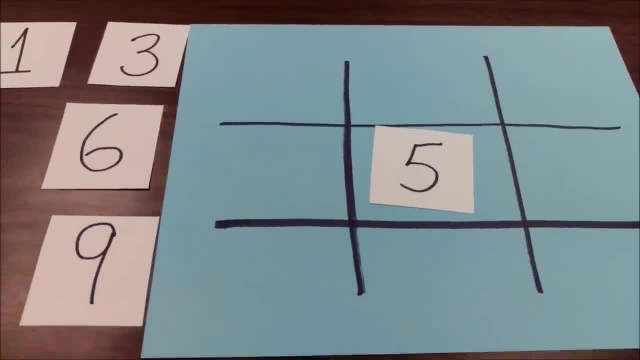 And you can go ahead and do that. You can ask Mr Hino, why can you not put a 5 in the middle? Because if you do, it guarantees that you're going to win. I don't know, it's kind of like cheating. 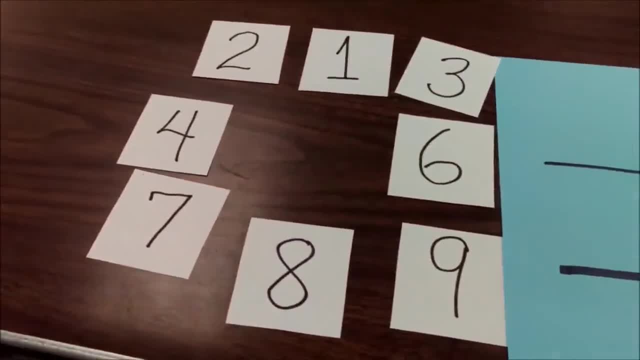 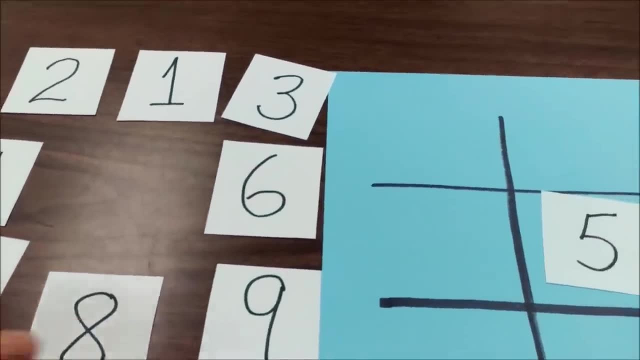 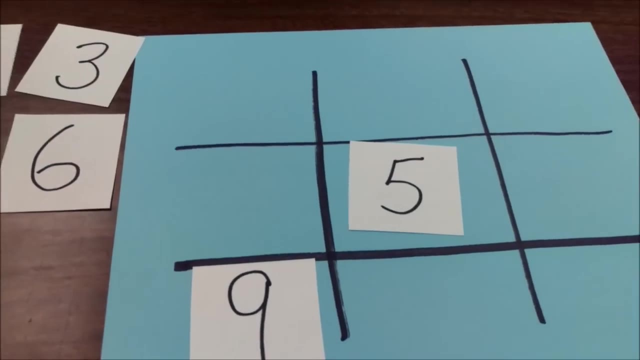 Because, look, if you put a 5 in the middle and the next person puts a number, there's nothing they can put that keeps you from not winning. if that made sense. I mean, look, if you put a 9 here, then the next person that puts a number, all they got to do is put a 1 up here. 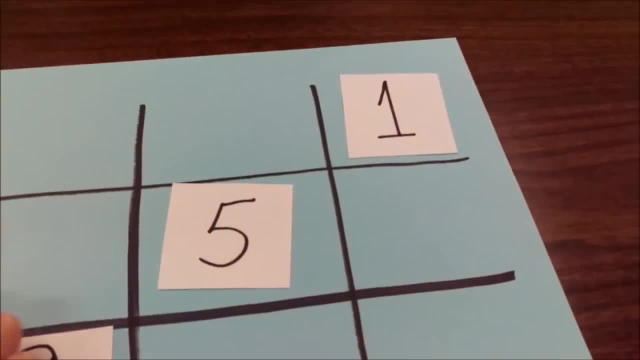 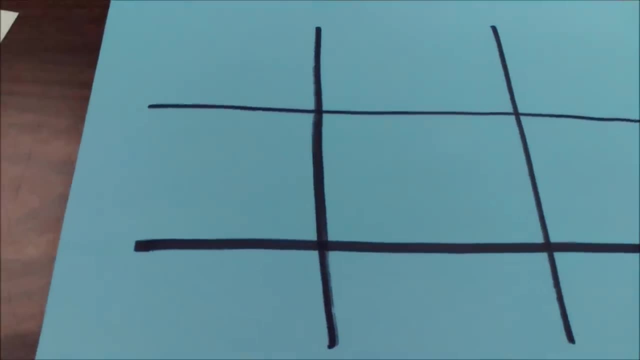 And they win. That equals 15.. So that's one of the rules: You just cannot put a 5 in the middle. to start with, You can put a 5 anywhere else, but you just can't put it in the middle. 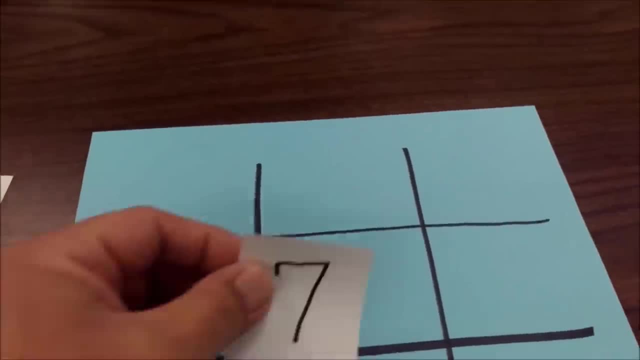 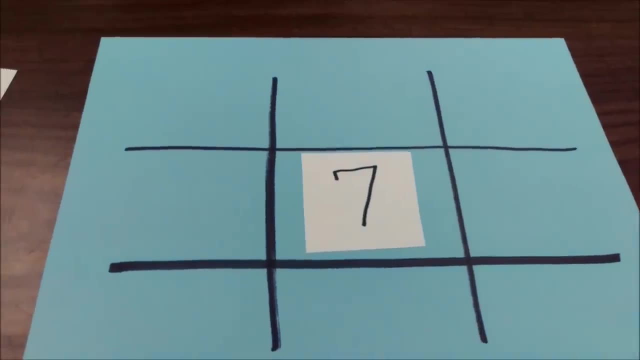 So let's just pretend we're playing a game. So let's say I go first and I put a 7 in the middle. Strategy would say: well, I have to make sure I don't put a number, if I'm going to put a number in. 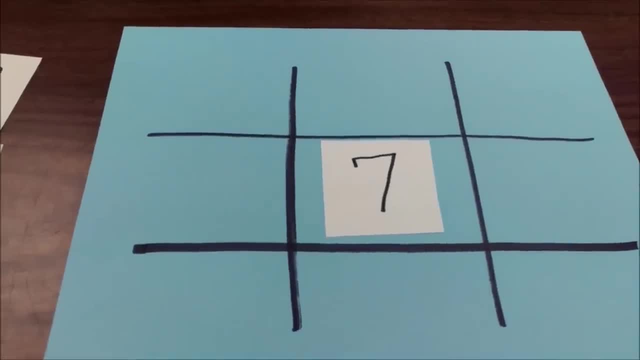 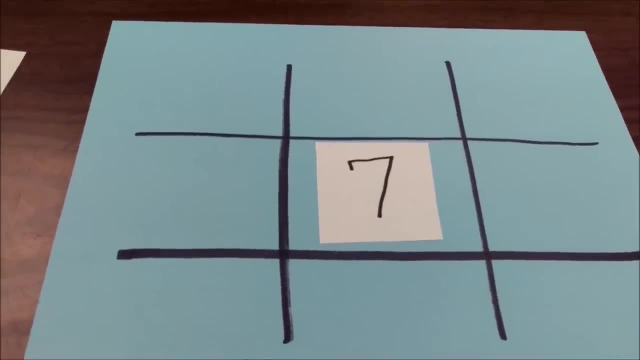 And right now, if I put a number, I'm going to have to put a number down in 7's column row or diagonal, because there's just no way around it. So one strategy would be okay. I'll put a 9 here. 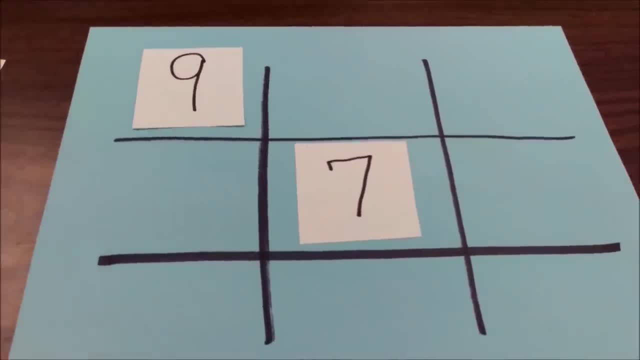 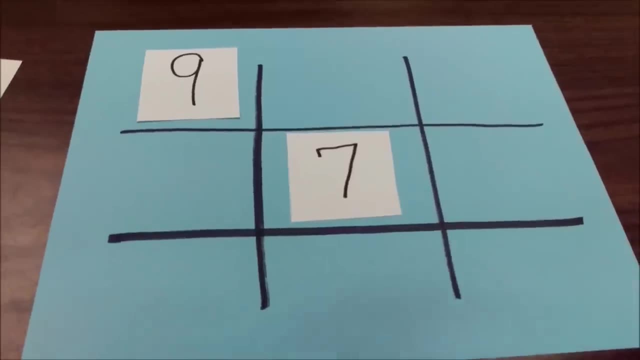 Obviously, 9 plus 7 is 16, and that's over 15.. So there's no way that I can win placing a number down here. So strategy would say: okay, I'm going to make sure that the person doesn't win for whatever number I put. 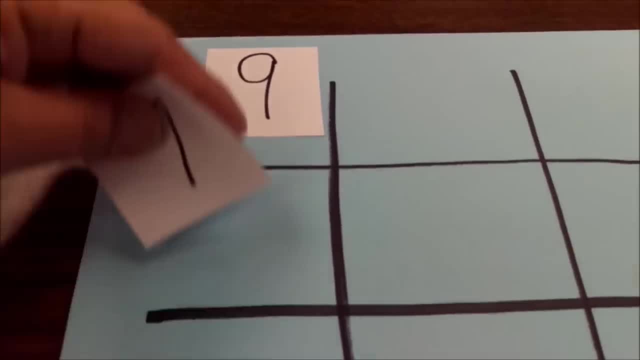 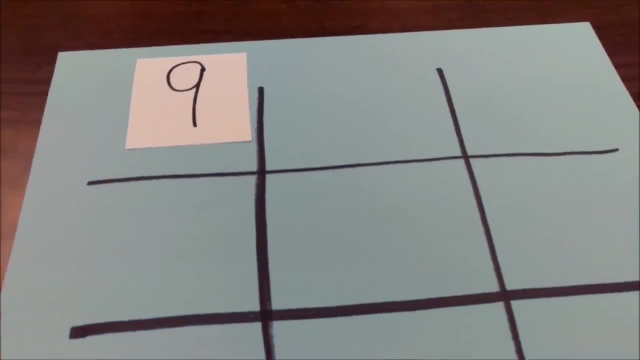 So this is just a cool game to play. You don't have to have people cut out numbers like this. You can just draw a tic-tac-toe and just know what numbers you have left, And again it's numbers 1 through 9..